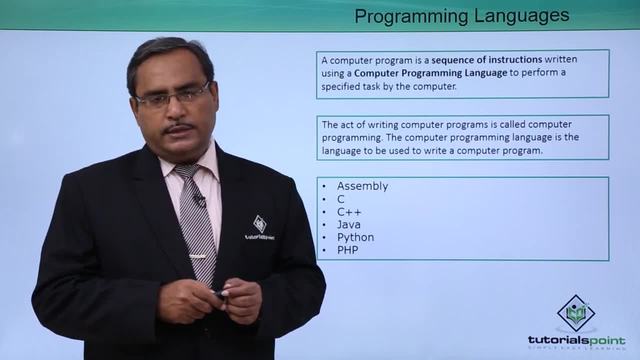 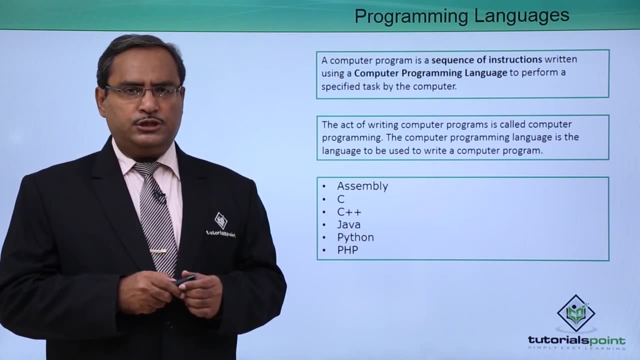 The computer programming language is the language to be used to write a computer program. So here we are, having so many different types of programming languages with the help of which we are able to write a computer program. Now let us discuss the computer programming. 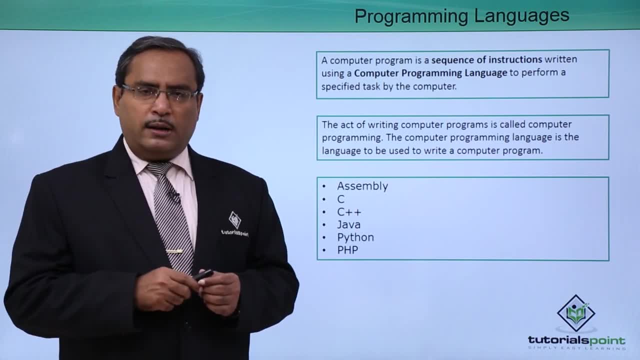 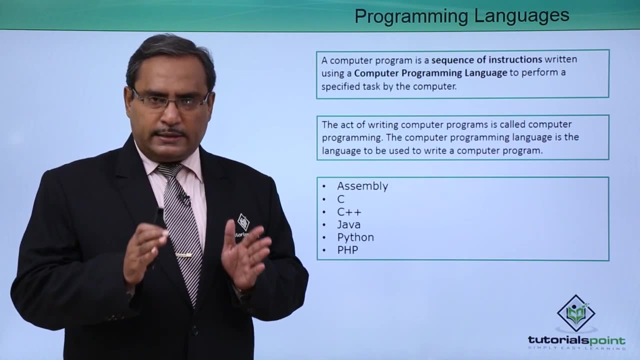 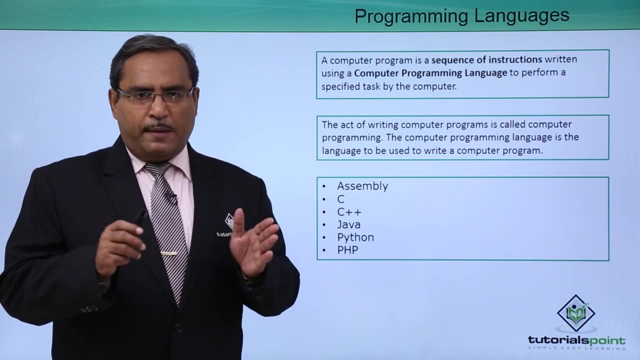 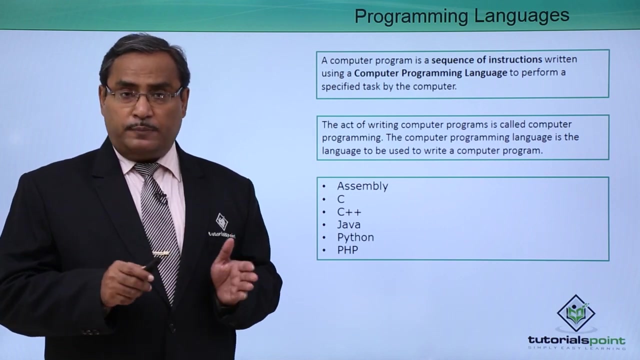 we can write computer programs, each and every program has got a separate syntax, then meaning of this term syntax is grammar, and they will be having a separate set of keywords with the help of which the programming can be written. different programs are having different purposes, different field of applications where this program will be used. so as a result of that, 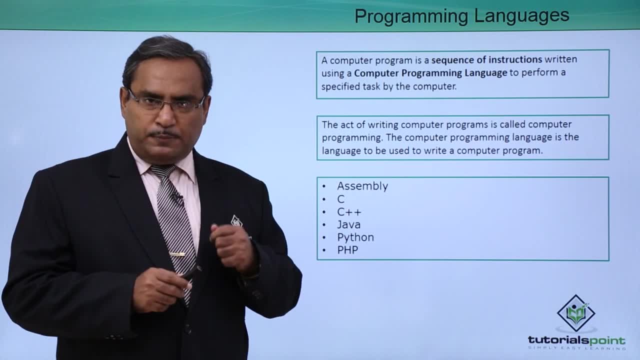 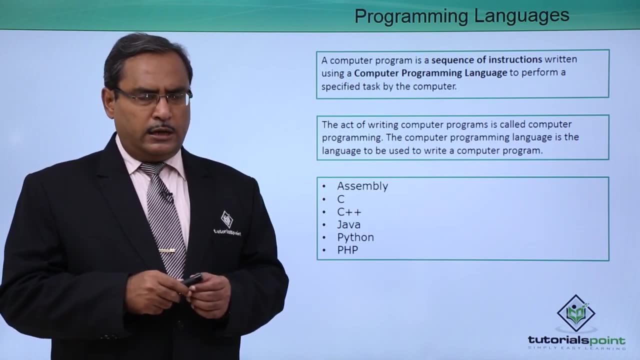 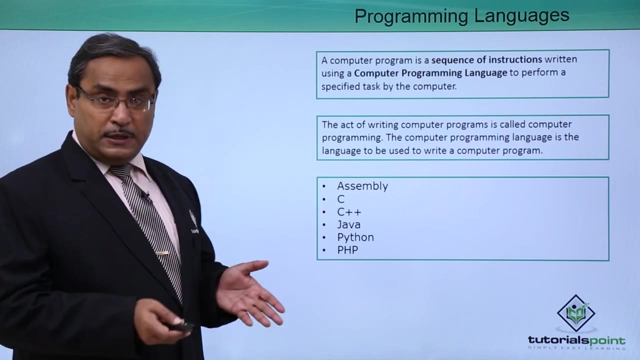 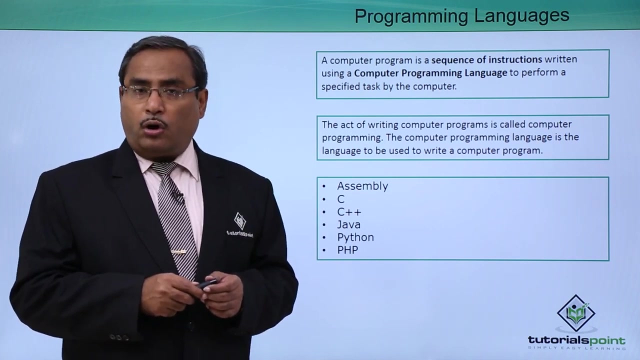 depending upon the nature of the application, we shall have to select and decide that what will be the programming language to be used to do the programming. nowadays, we are having so many different languages, like our assembly level language, we are having c language, c plus plus, on which we are doing this tutorial, and java, python, php, pearl, kotling and so on. 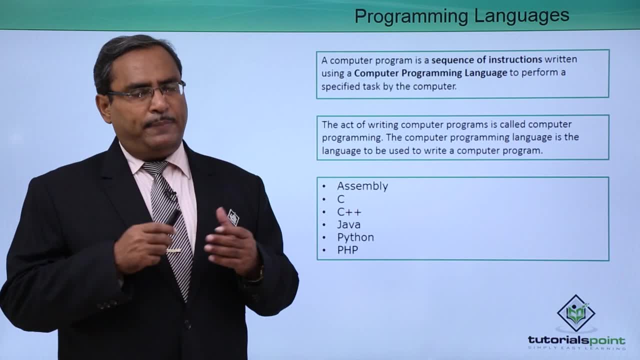 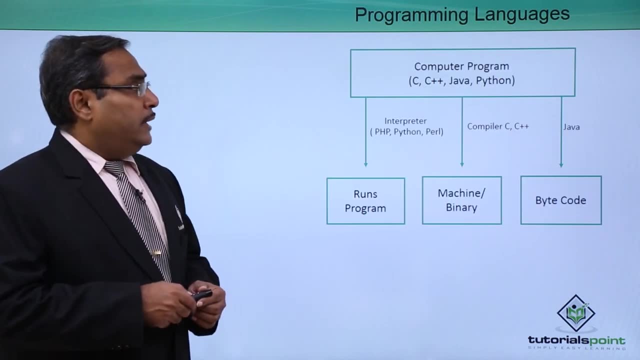 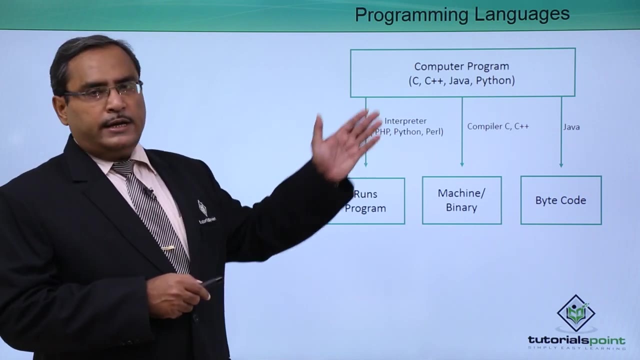 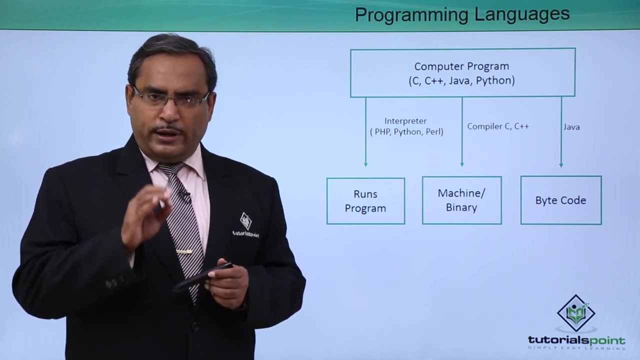 so each and every language has got its own domain of application and a separate set of keywords and the respective syntax. a computer program, let it be c program or c plus plus java or python program, and they will be written in some high level language. high level language means the language in english like language. so where we will be, 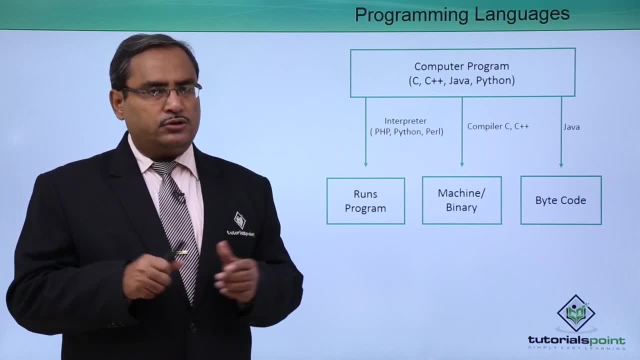 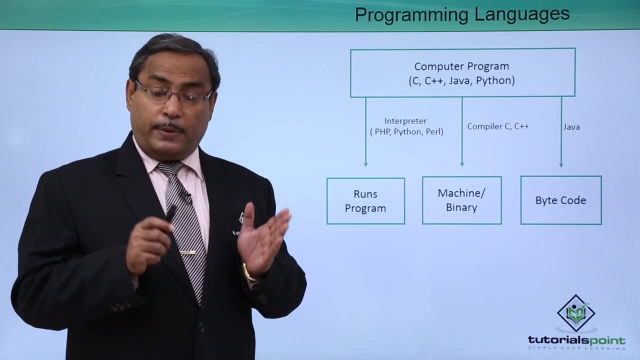 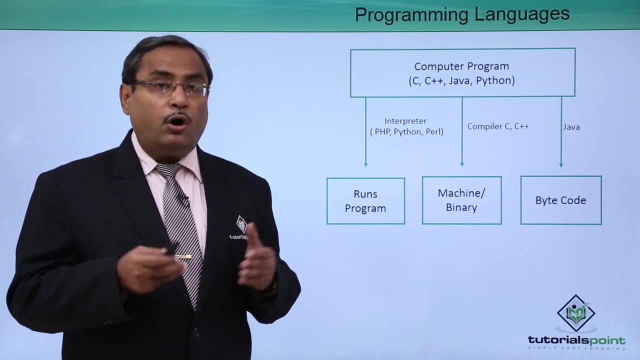 writing our program in english alphabets because on the keyboards we are having the english keys there. english alphabet written keys are there on our keyboards but computer can under cannot understand this one. so computer can understand only the language of machine language or low level language. so as a result of that we require some translator which will translate this high level language. 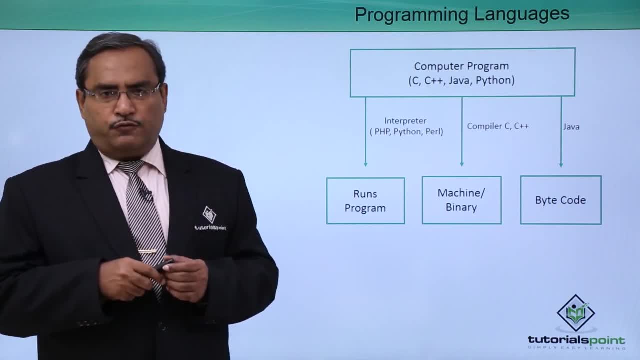 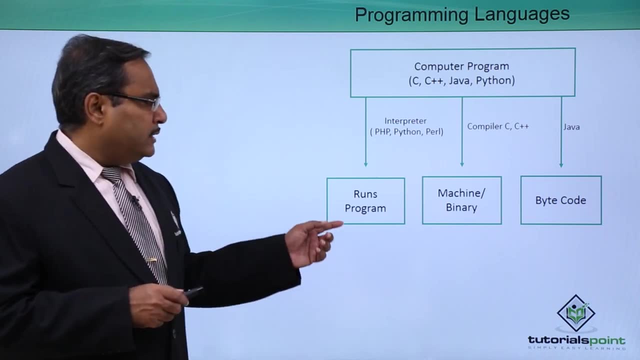 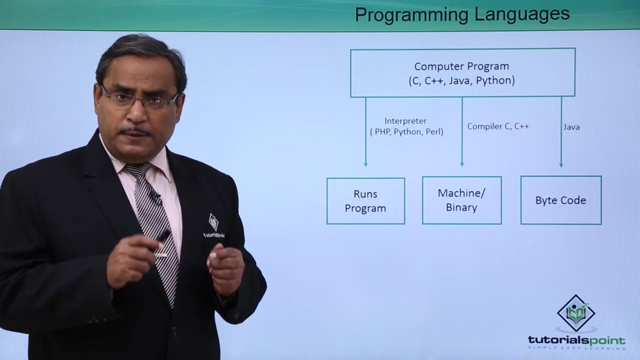 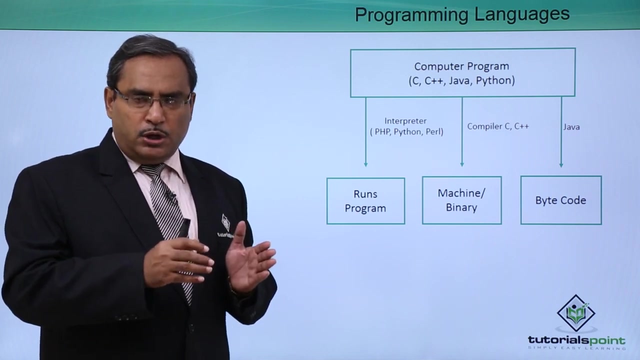 program to the respective low level language program. so for different types of languages, programming languages, we are having different kinds of translators. so let us suppose for, say this, I have php, python and pearl. we are having interpreters. interpreters are nothing but a separate program which will do the translation of the high level language program to the 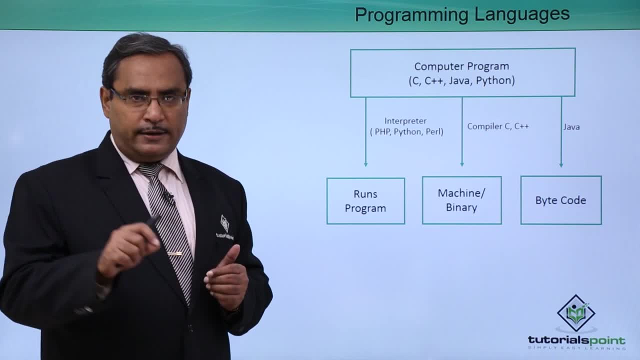 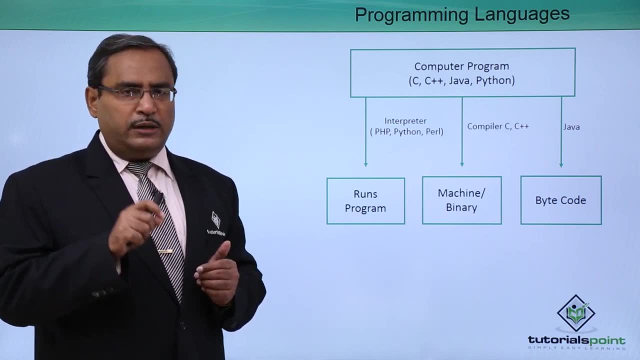 machine level language or low level language, line by line. that means prior execution of each and every line of the main code. the line will be translated to the corresponding machine code and the code will get executed. if the line gets executed for 1000 number of times, 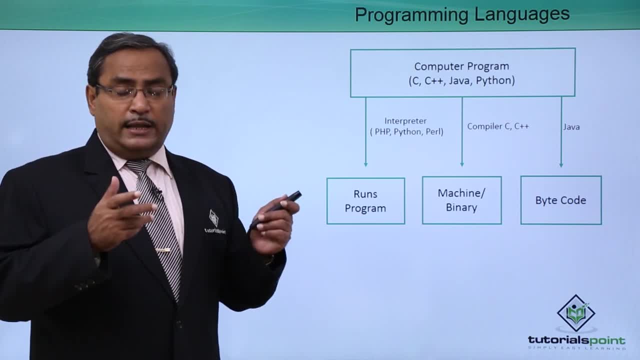 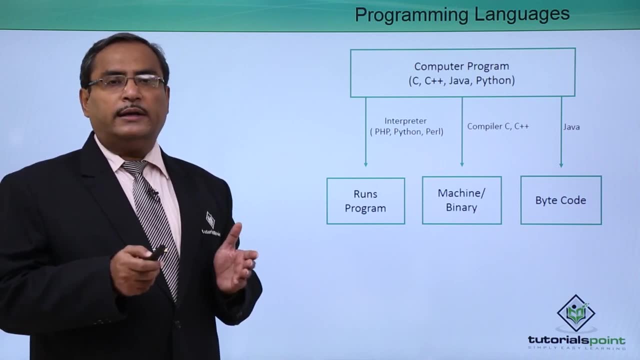 if the line is in a loop, then in that case that line will be translated for 1000 number of times in that case. so that is the purpose of interpreter. so interpreted is one kind of, one kind of translator which is transferred from high level language program to the machine. 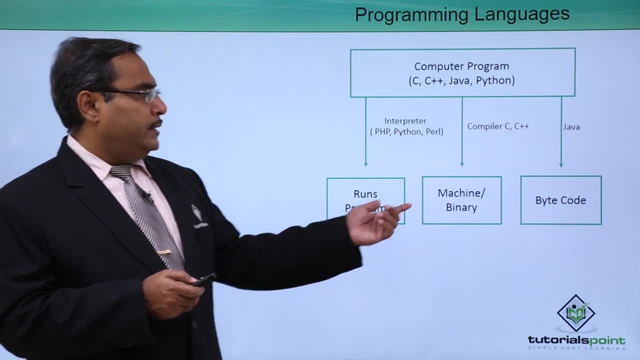 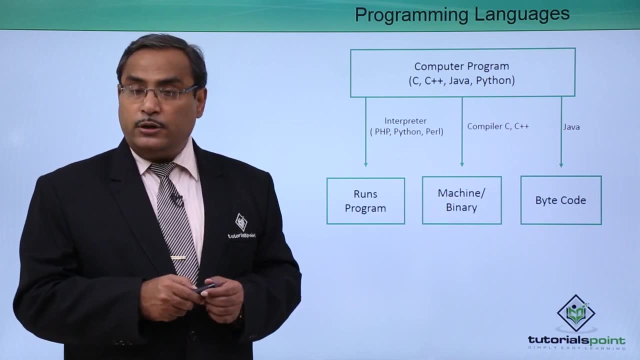 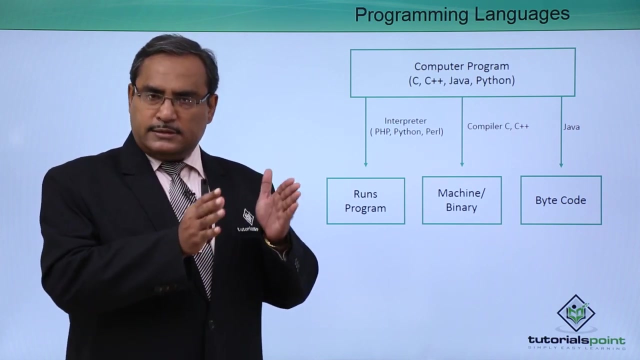 level language and it runs the program in this way. we are having this c and c plus plus. we will be having our compilers and it will produce the machine or binary code, language as output. and here, with what, what it will happen? the main program will be written in certain language. let it be in C or C plus plus. then 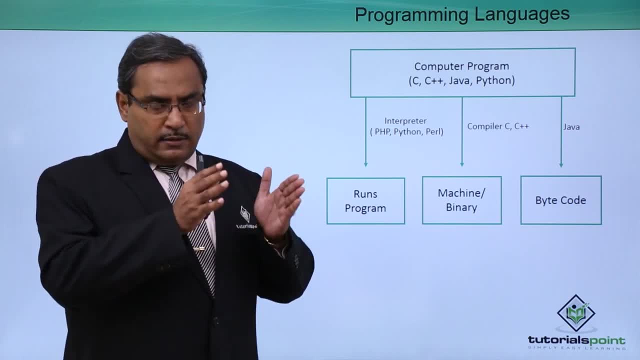 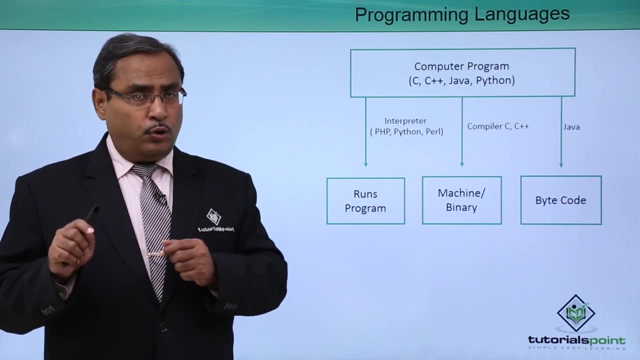 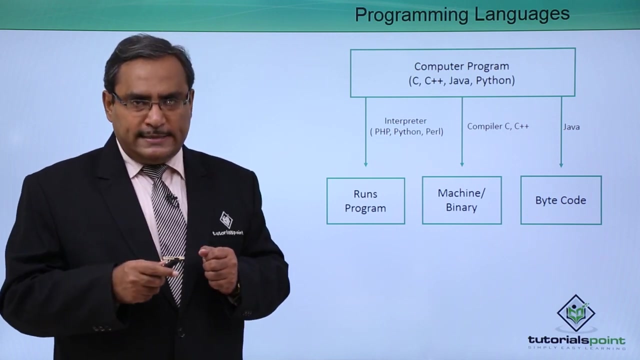 compiler will come into the play which will translate this high level language program to a separate file, which will be in binary language or machine level language, and that program will get executed. that compiled version of the program will get executed And in the system where that program will get executed- there we do not require the coexistence. 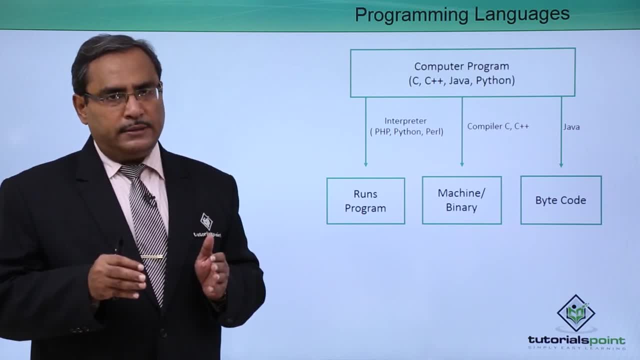 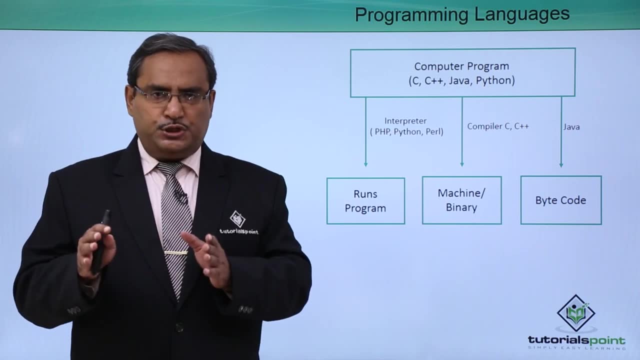 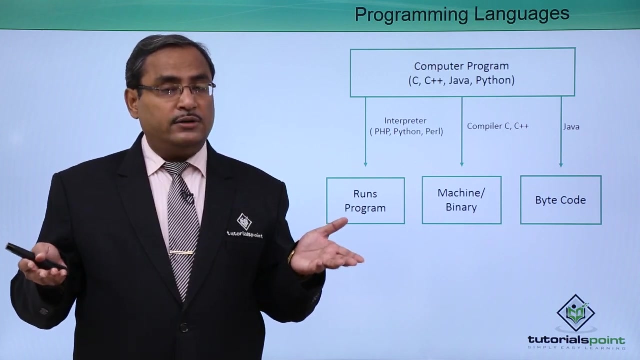 of the source code along with the compiler, because, ultimately, after being compiled, the executable version of the program will be self-sufficient, so that it can get executed in a system where there is no existence of the source code, written either in C or C plus plus, or the compiler software which will do the translation. 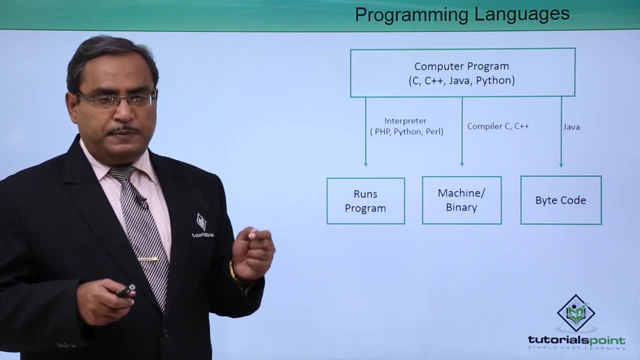 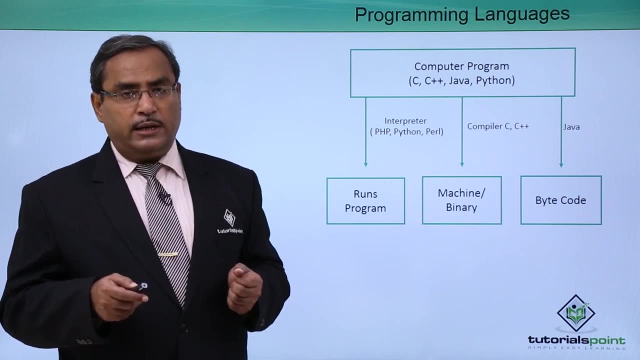 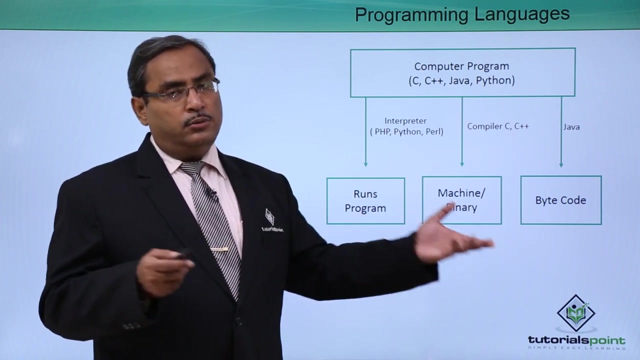 There is another way. in case of Java, we are having the respective translator, which will translate this Java source code into a binary Java byte code format and later Java virtual machine will come into the scene and which is platform dependent and that will convert, that will execute this byte code. written program. 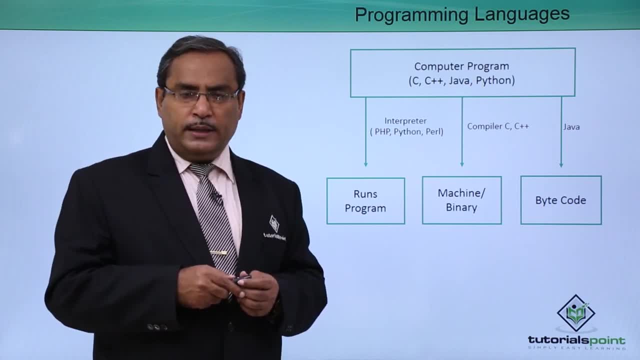 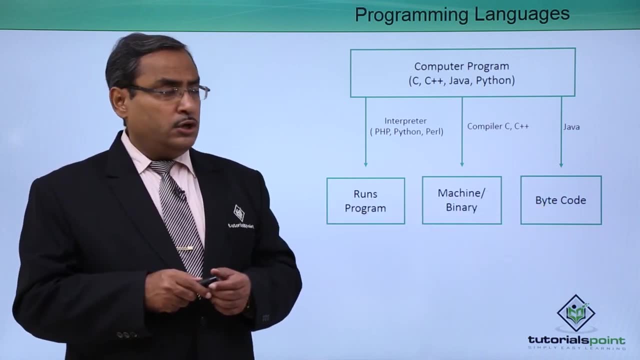 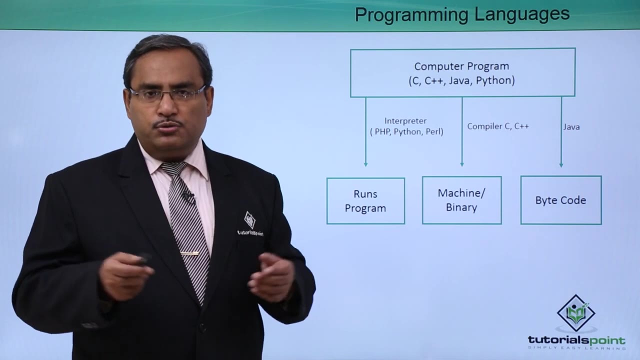 to the required execution and corresponding outputs will be produced. So this is the. this is the Java program which will be converted to the respective byte code format. So in this way we have explained that how the high level language program can get. it can get its execution through going through different translators. Thanks for watching this video.